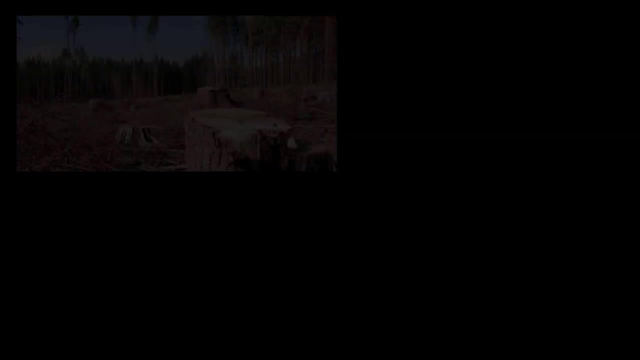 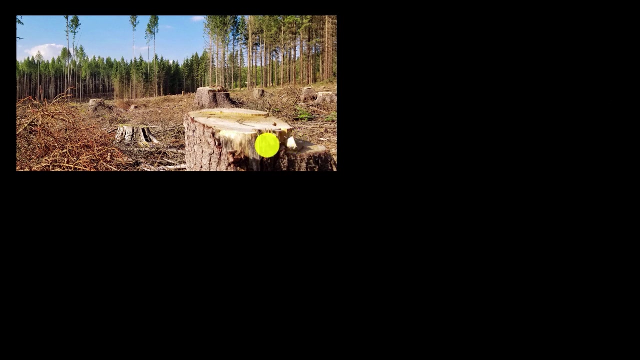 we'll think about it in five different dimensions. The first is habitat destruction. So this over here is a picture of some trees that have clearly been cut down, and there's many reasons why trees could be cut down like this One could be. maybe there's some logging here. and we human beings, we do need wood. Maybe it's being cleared for agriculture, which we also need, But when you do that, it's clearly eliminating the trees and many animals. many different types of species- were probably living in or amongst or on those trees. 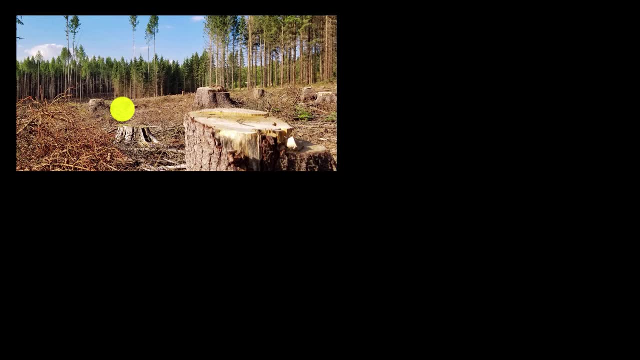 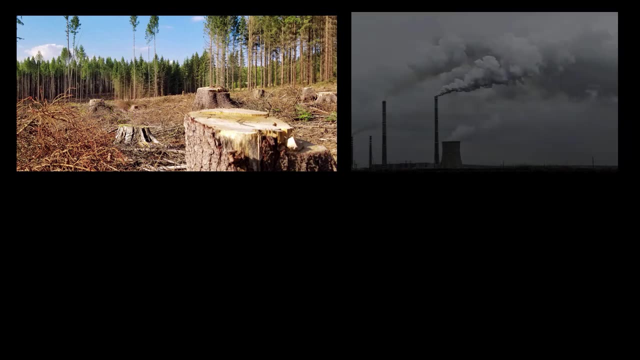 And if you do too much of that, they might not have anywhere to live or they might not have enough places to live to really thrive. Now, another form of anthropogenic changes or changes induced by human activity would be pollution. This right over here, you can see the exhaust. 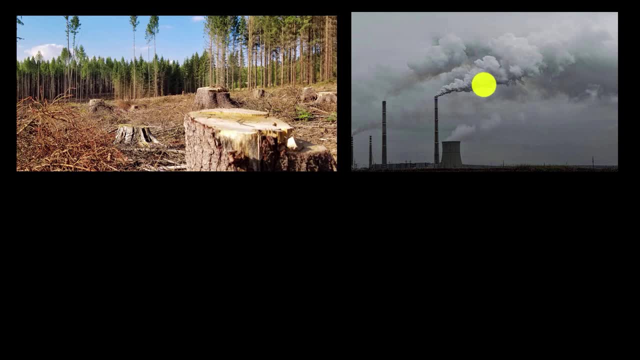 so to speak, from a coal-fired power plant, and that is polluting the air. Harmful chemicals are being released, including greenhouse gases, and that's going to have other effects above and beyond just making the air less pleasant. But pollution isn't just about harmful chemicals. 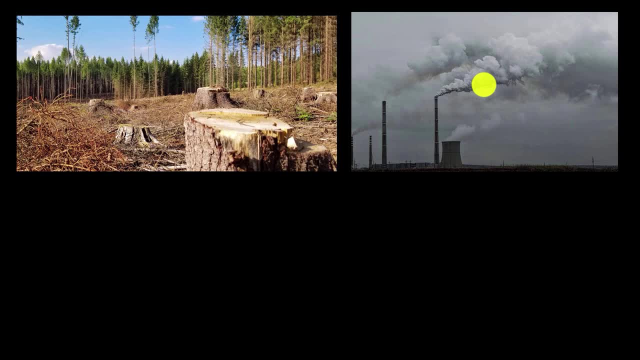 going into the air. It could be about harmful chemicals going into into the water. It could be runoff from irrigation or some other type of chemical. You can even have noise pollution and you might think of that as an annoyance, but it can actually disrupt how certain animals behave. 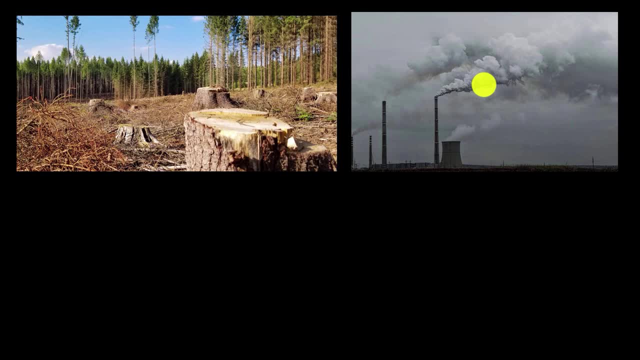 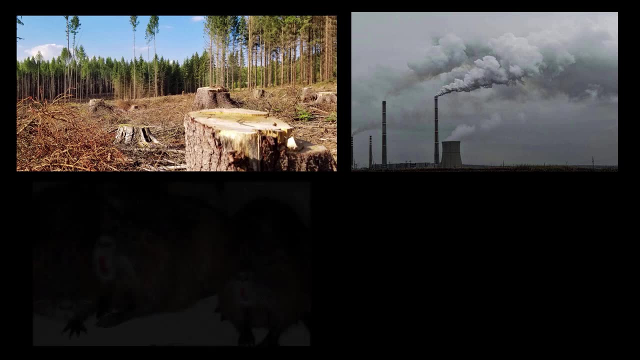 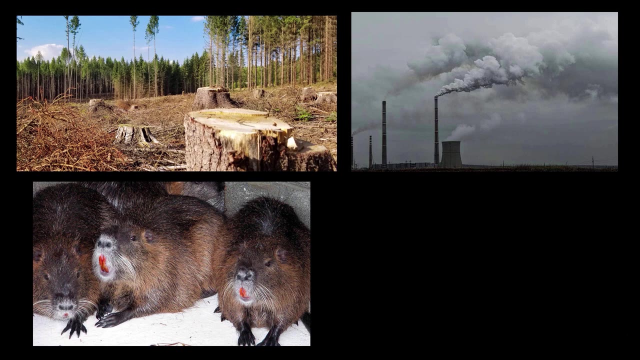 In fact, it could raise the stress level, which can change the biology of animals in subtle but important ways. Another dimension in which we humans are affecting ecosystems is by introducing species to places where they might not have been before, especially what's often called invasives. 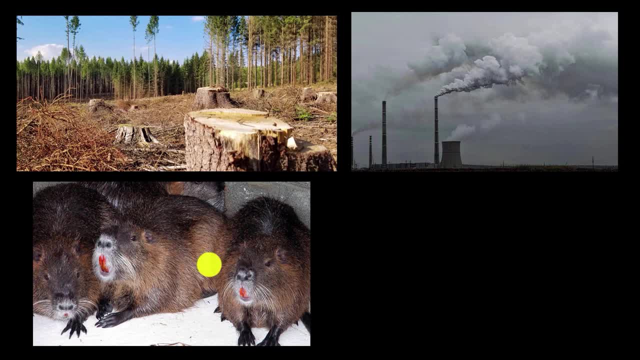 native species. So this is a picture here of nutria, oftentimes referred to as nutria rats. I was born and raised in Louisiana and there are many nutria in Louisiana and they did not come from Louisiana. They came originally from South America. 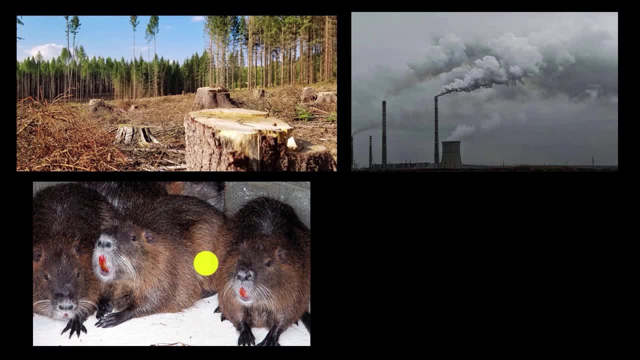 They were brought to the Gulf Coast, to the southern United States, for their furs. The demand for their furs did not keep up and these nutria escaped, and now they are everywhere, And you might just once again view that as an annoyance. 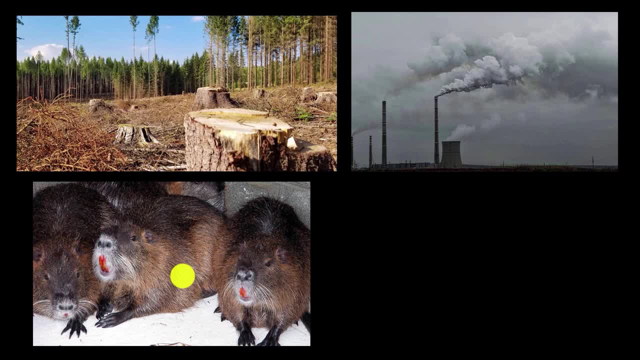 but they start overpowering other species. They are competing with other animals for the same food, for the same niche in the ecosystem. Nutria are also infamous for eating the plants that hold together the soil and the wetlands, And so the more that they do that. 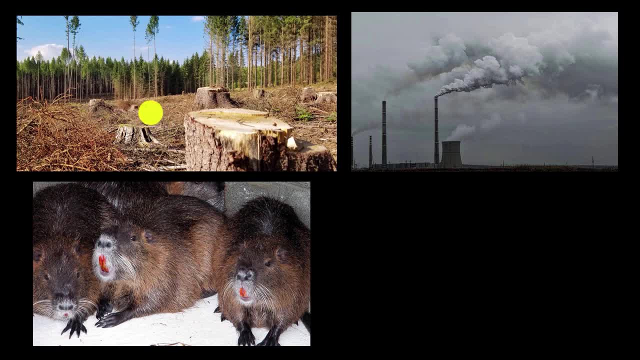 the more that that soil gets eroded, And then you have issues like habitat destruction. You have fewer wetlands for other species. Now, another dimension is over-exhaustion Exploitation. So this is a picture here of what's known as trawling. 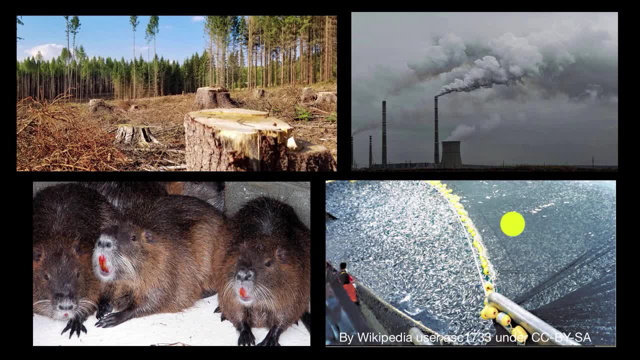 where you take a big boat and you have this huge net and you just the boat goes while the net is just grabbing all the fish in the water And these dots here are all fish and actually it extends out here because the net is bulging outward like that. 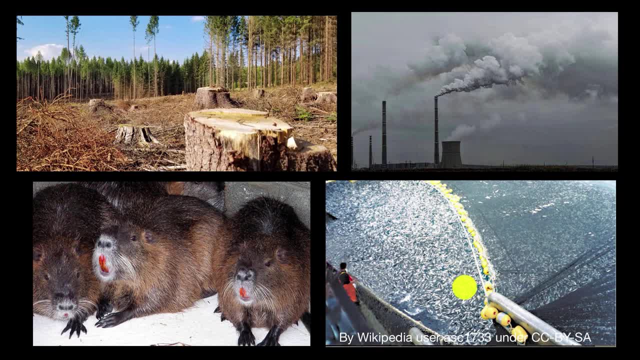 And you can see. it's a very efficient method of getting fish, but you could over-fish. If you take too many fish out of the ocean, you're not going to have enough to reproduce and keep the population going, And even though you might get a lot of cheap fish, 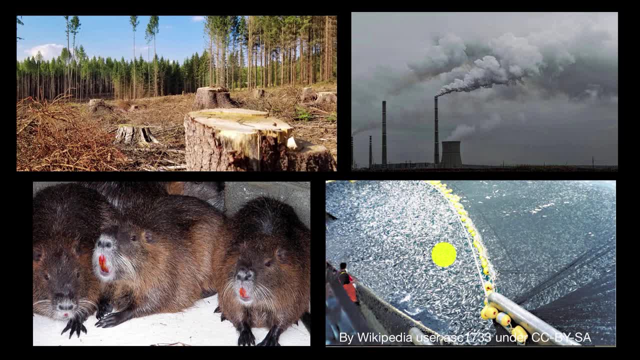 very efficiently in the short term. in the long term, the fish might go away. All of these, as you can imagine, connect in many ways, And a fifth dimension we could talk about, although it's very related to pollution and even deforestation, is climate change. 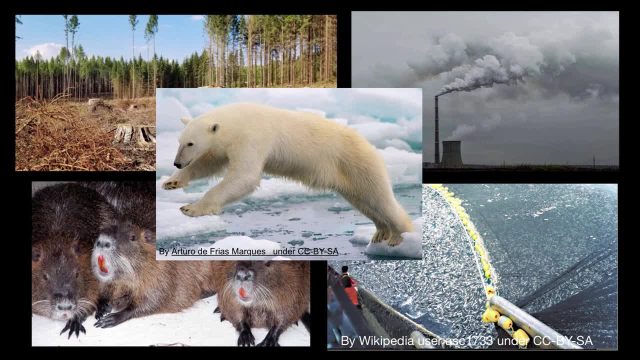 And the climate change that we are most familiar with right now is this notion of global warming, which is occurring as we have rising levels of greenhouse gases like CO2, and those could be released from things like this coal-fired power plant that we saw a few minutes ago. 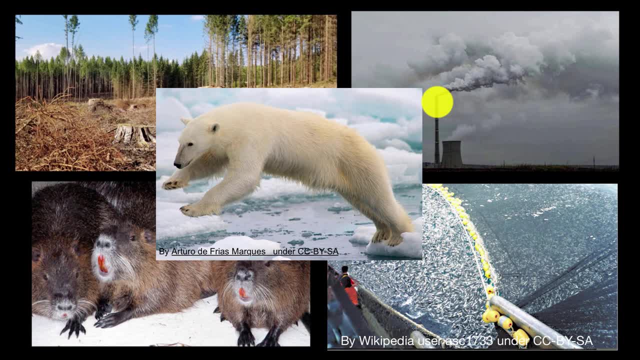 But there's many other sources of things like CO2, and there's other greenhouse gases. But as we human beings release more and more of this into the atmosphere, these greenhouse gases trap more and more heat, And that over the long term. 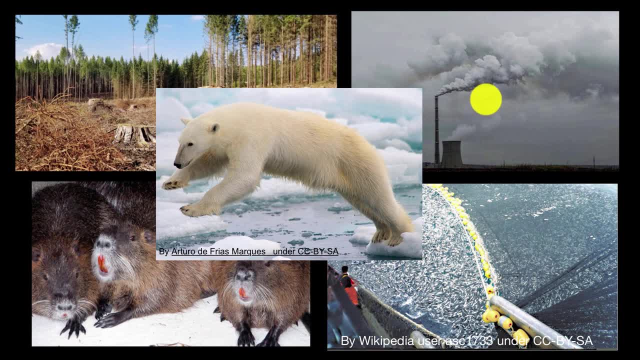 increases average global temperatures, And that doesn't just affect temperature. When you affect temperature, it can affect rainfall, it can affect wind patterns And, as we see in this picture over here, it can affect things like the amount of sea ice we have. 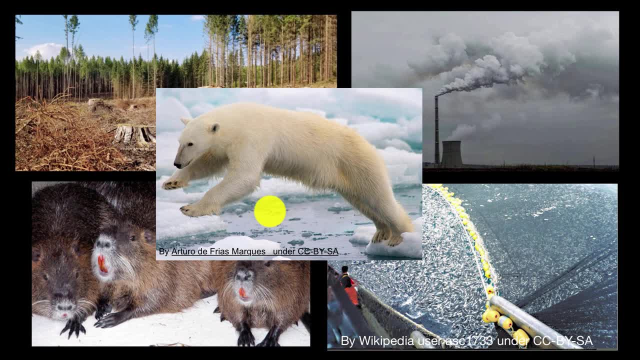 because if, on average, global temperatures are increasing, then water temperatures could be increasing. Then you have more melting sea ice in both the Arctic and Antarctic And then, for example, in the Arctic, where you have polar bears, they would have less ice to be on.